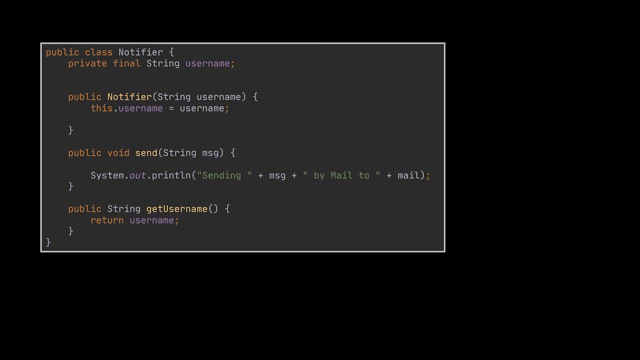 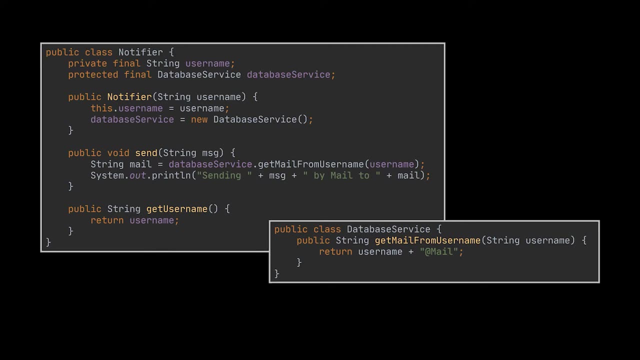 method. this method could accept a message argument and send this message to an email which is retrieved from the username via a database service class. now, at some point, you realize that our customers expect more than just email notifications. many of them would like to receive a whatsapp message about their deliveries, for example, and others would like to be notified. 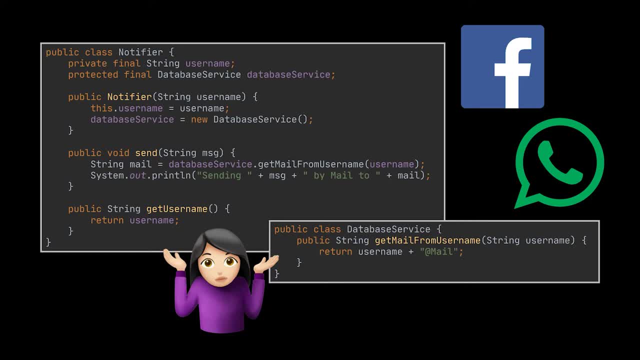 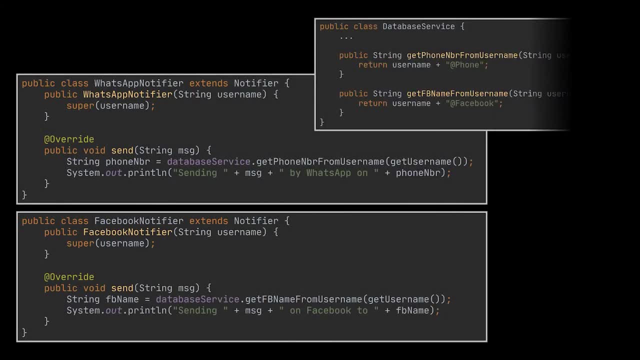 via facebook. how hard can that be right? and the first thing that comes to mind is, of course, inheritance. so you extended the notifier class with two new subclasses: the whatsapp notifier and facebook notifier classes. now the client is supposed to instantiate the desired notifier class and use it. 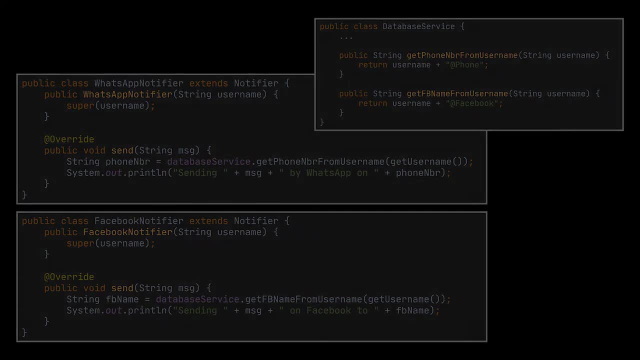 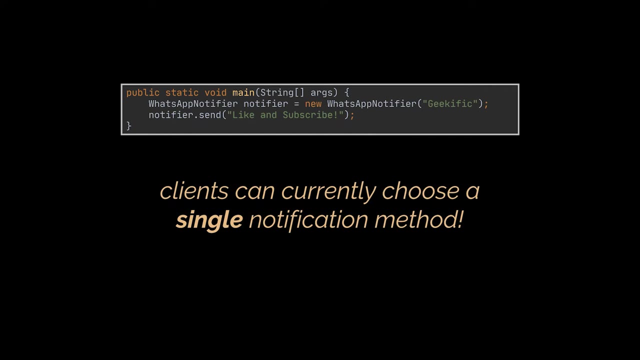 while notifying a particular customer. however, one day, one of the customer approaches you politely and says: why can't i be notified via whatsapp and facebook at the same time? well, with the current design, the solution to this problem would be to create a new class that would be able to. 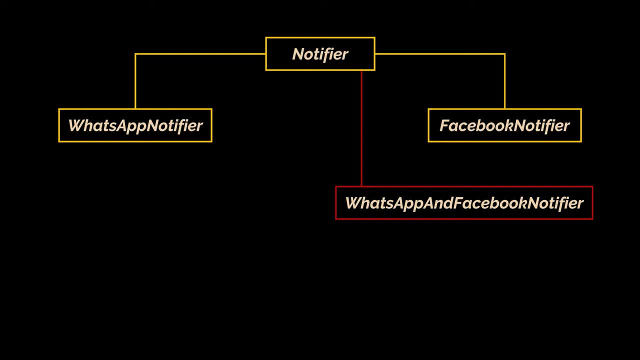 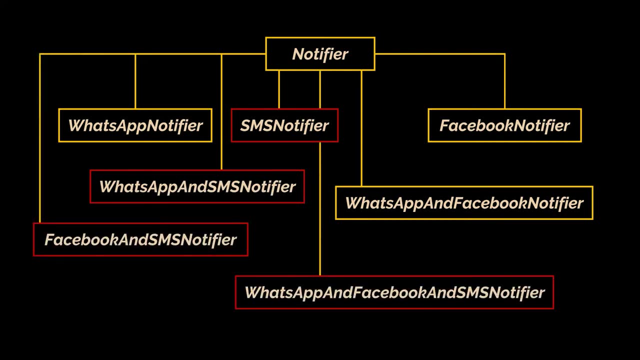 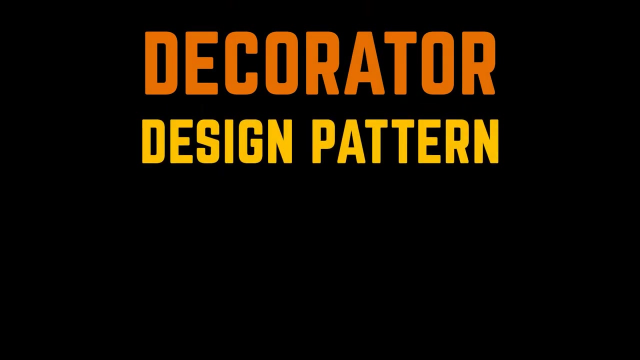 notify this customer using both facebook and whatsapp, but notice how this approach would overwhelm the code immensely. when you try to add a third notifier, like sms, for example, you can clearly see that by adding this single additional choice, the number of subclasses we have are already hard to keep track of. the solution to such problems is following and applying the decorator. 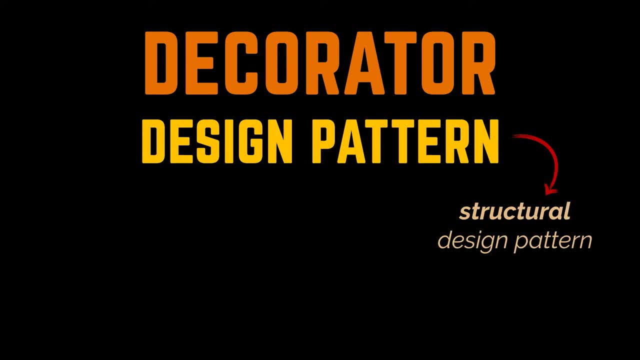 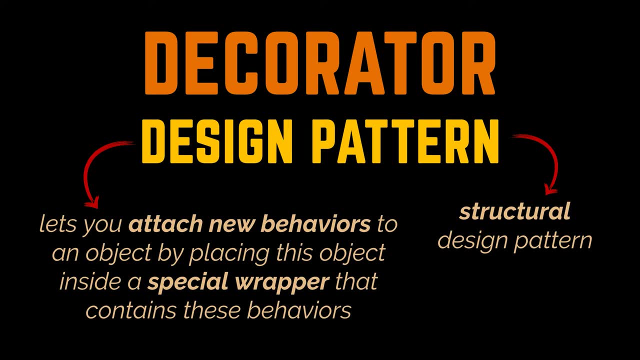 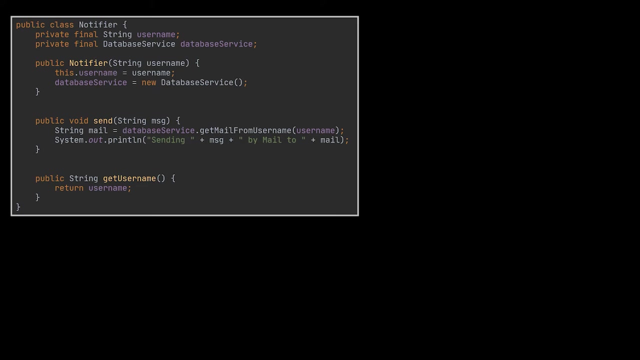 design pattern. the decorator pattern is a structural design pattern that is used to attach new behaviors to an object by placing this object inside a special wrapper object that contains these behaviors. let's try to apply that on our notification service example. to do that, we will keep the main component of our app, the notifier class, intact. however, concerning the 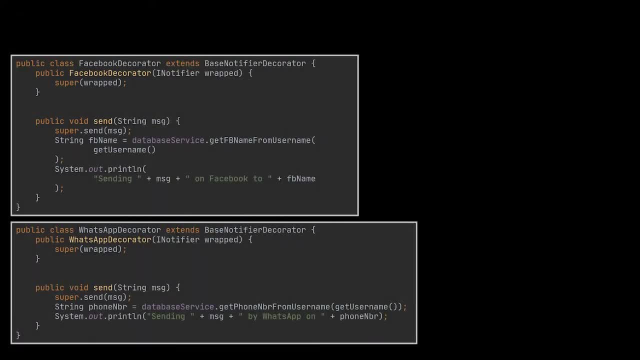 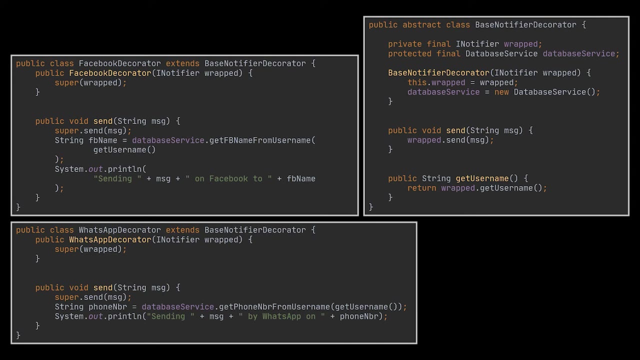 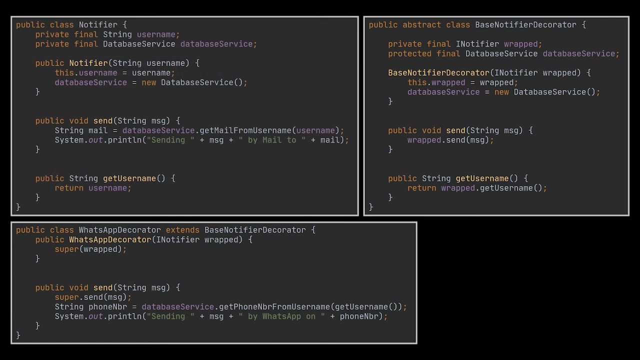 facebook notifier and whatsapp notifier classes. these classes will be renamed to facebook decorator and whatsapp decorator and will now extend a base notifier decorator class. this base decorator class is the wrapper or the container of our initial notifier. the next and most important step is to make all the classes. 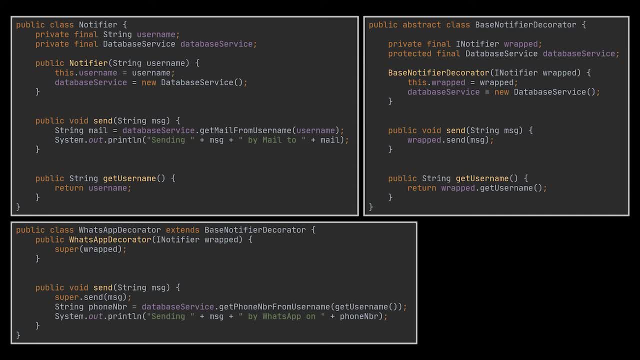 we just saw implement the same interface- let's call it i notifier- and it is this interface that will be used by our classes across all our application, and by the wrapper class as well. why is that? well, to understand this, let's take a step back and take a look at the decorators definition. 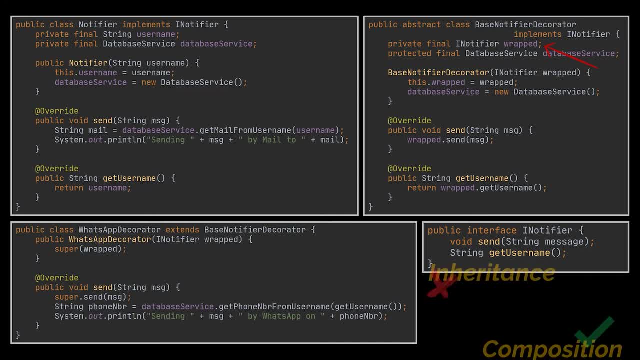 mentioned a few seconds ago. we said the decorators are wrappers for our core objects, and wrapping enforces us to replace the inheritance we've been using with composition. an advantage of composition is that you can easily substitute your objects with one another, because all of them belong to. 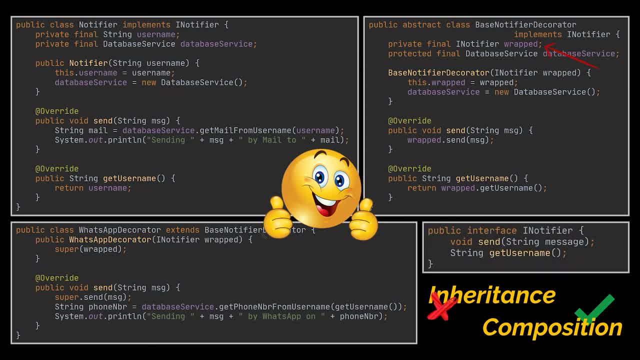 the same interface. this allows you to change the behavior of the container at runtime. on top of that, an object can use the behavior of various classes, not only one, as it can reference multiple objects and can delegate them all kinds of work. now the rest of our code won't care whether it works with the initial notifier object or the decorated. 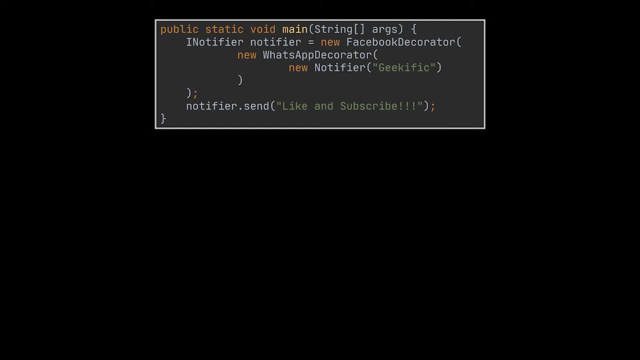 one, since all decorators implement the same interface, as does the base notifier class. as you can see, in this example, the wrapped object provided to the facebook decorator is itself a what's up decorated one, which was provided with a simple notifier, meaning that the facebook super dot send method call will invoke the whatsapp super dot send method, which 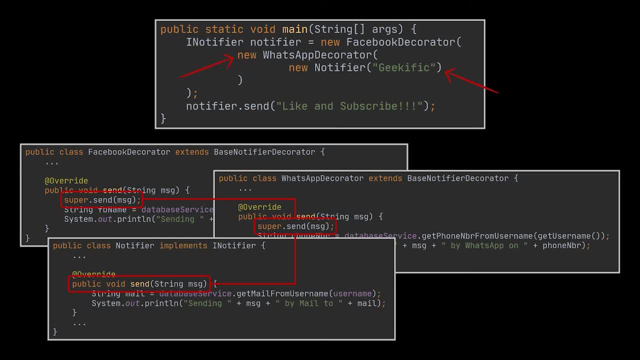 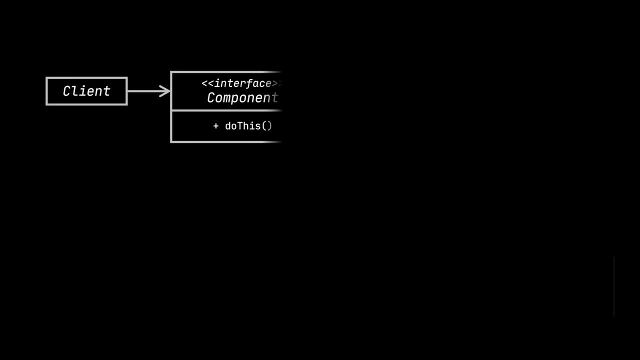 will invoke the base email notifier send call leading to the output you see in front of you. okay, now that we've implemented and applied the decorator pattern, let's take a look at its structure or class diagram, all while trying to relate it to the notification example we 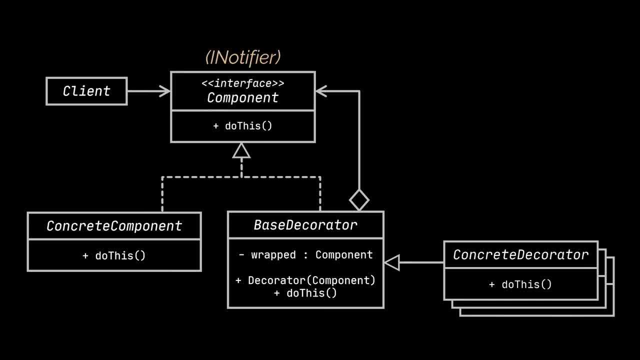 just saw. the first thing you may have noticed is the component interface, which was represented by the i notifier interface in our example. this interface declares the common behaviors for both wrappers and wrapped objects. next is the concrete component, which, of course, was the notifier class in our example. this is the wrapped class. it defines the basic.